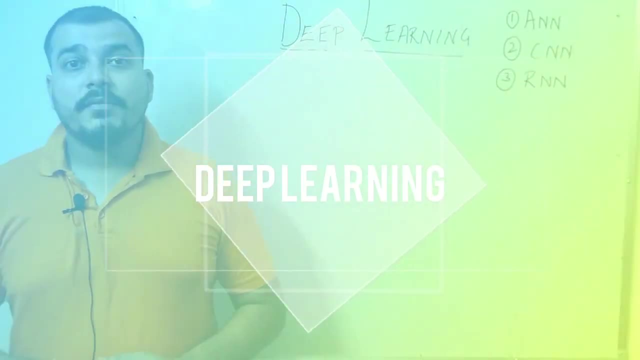 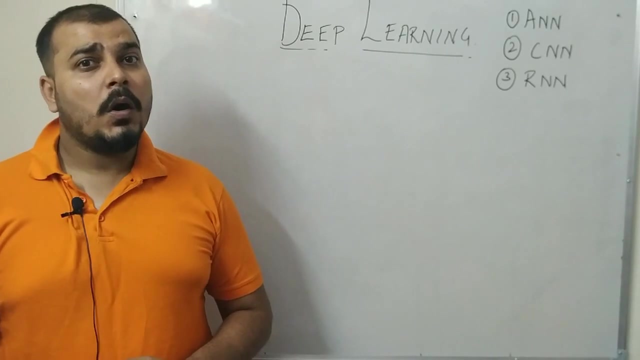 Hello all. my name is Krish and welcome to my YouTube channel. In this particular video, I am going to create a playlist on deep learning and wherein I will be explaining all, everything: all the concepts in deep learning and all the different types of neural network models and architecture. 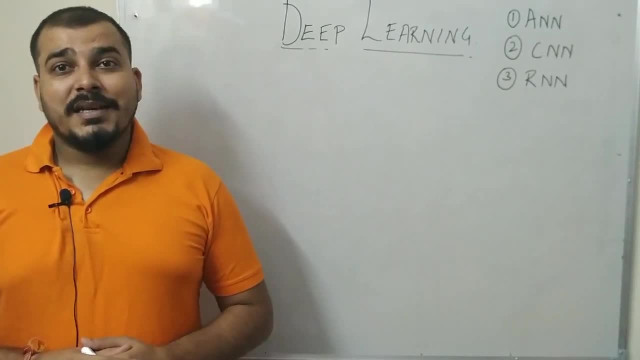 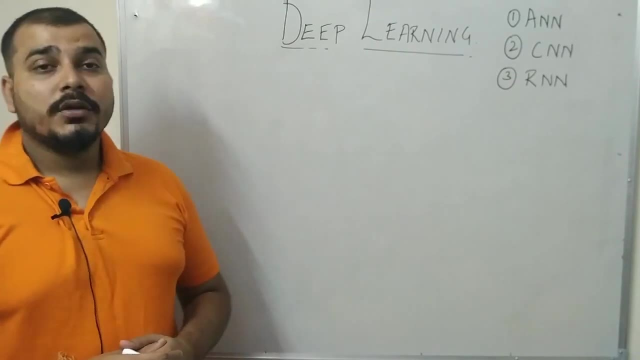 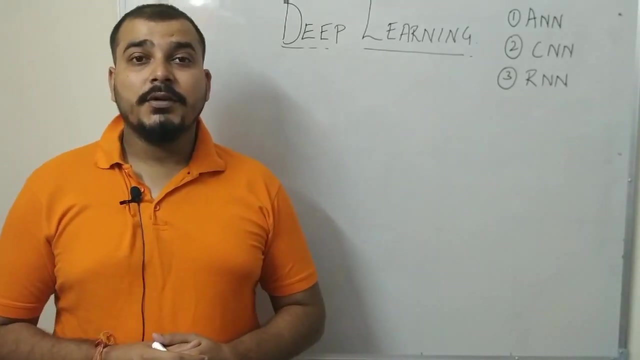 This particular playlist was basically requested by most of my subscribers to explain everything of deep learning from scratch. So the first topic that we are going to basically discuss today is basically about the neural network architecture, and then we will be discussing some of the base models like artificial neural network, convolutional neural network and the RNN that is called as recurrent neural network. 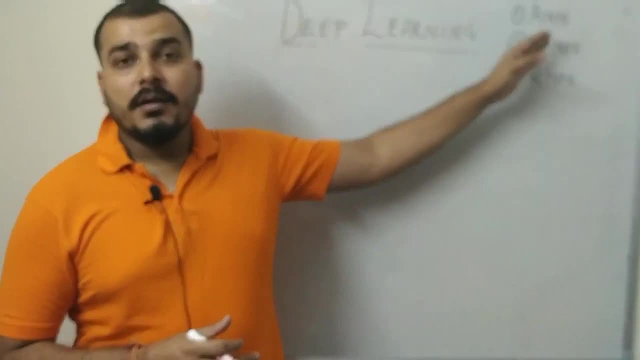 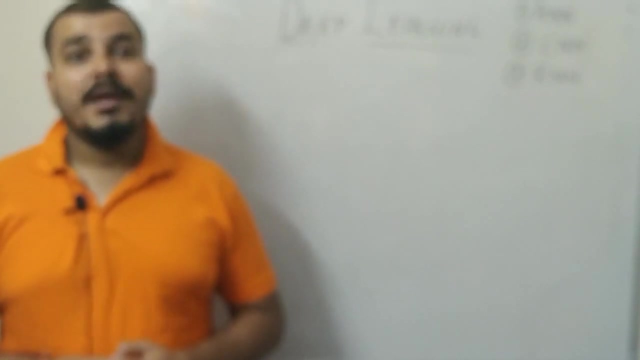 After this gets completed. so as soon as I complete the theoretical part of artificial neural network, I will also be showing you the practical implementation with the help of the artificial neural network. I will also be showing you the practical implementation with the help of various libraries like TensorFlow, Keras and PyTorch. I will be taking the use cases from Kaggle and I will be solving all these particular use cases. I will be uploading all the code in the GitHub. So please diligently follow this particular playlist if you want to become a pro in deep learning- and you want to. you know, if you are planning to switch your jobs, it will be definitely really helpful. 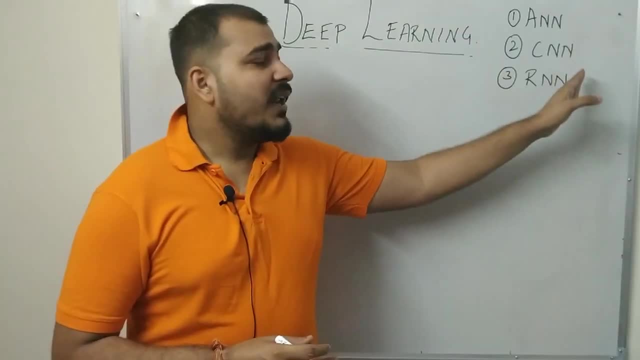 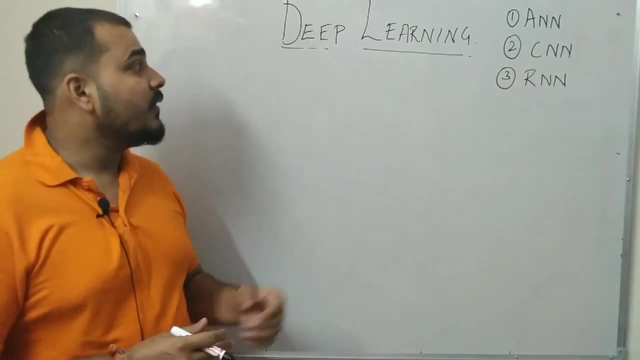 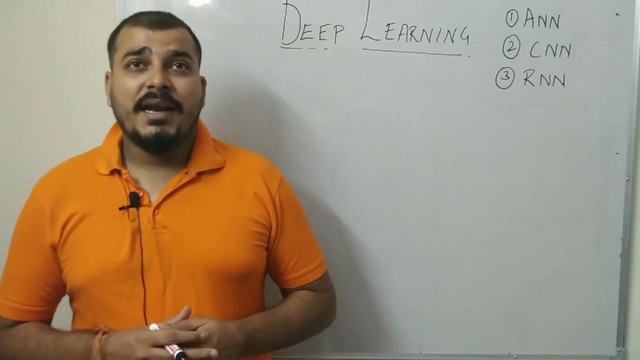 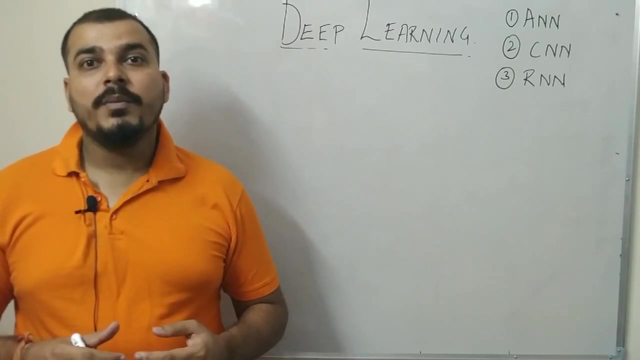 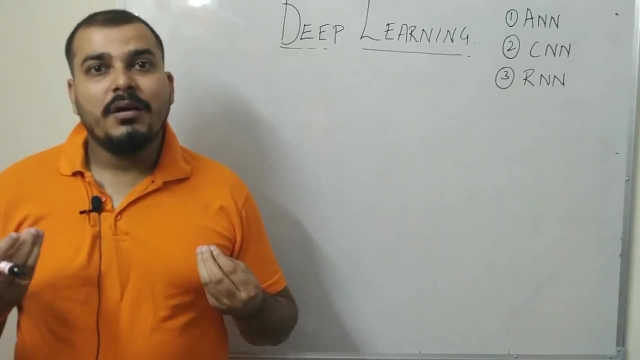 So let me just discuss about ANN and CNN, RNN, because these are the base models. first of all, Before going ahead in understanding ANN, CNN and RNN, we will first understand what exactly is ANN and CNN. So ANN and CNN, RNN is basically deep learning. So deep learning is a technique which basically mimics the human brain. So in 1950s and 60s researchers and scientists thought that can we make a machine learn and work like how we human actually learn? and you know that we will be learning from the, basically from the environment, with the help of our brain. you know our brain has such a capacity that it can learn various things very quickly. 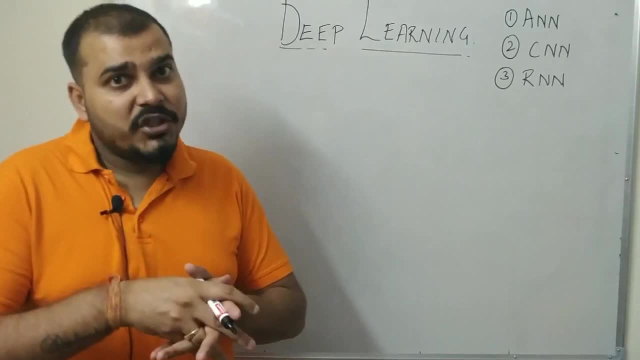 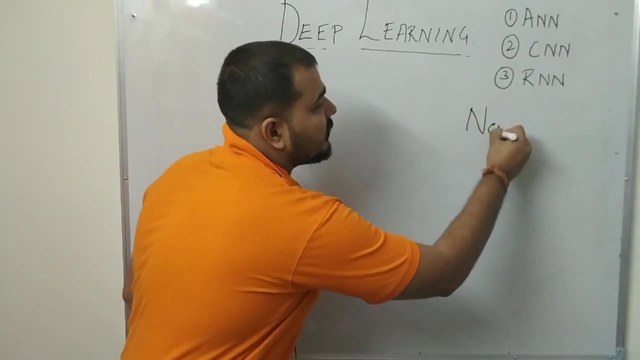 So the scientists and researchers thought: can we make the machine learn in the same way? So there is where the ANN and CNN RNN came from. So that is where the deep learning concepts came and that led to the invention of something called as Neural Networks. Neural Networks. 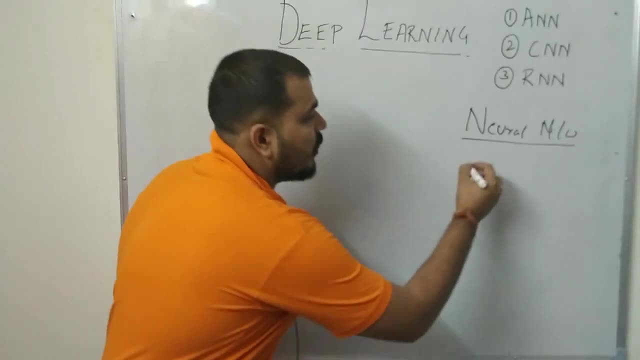 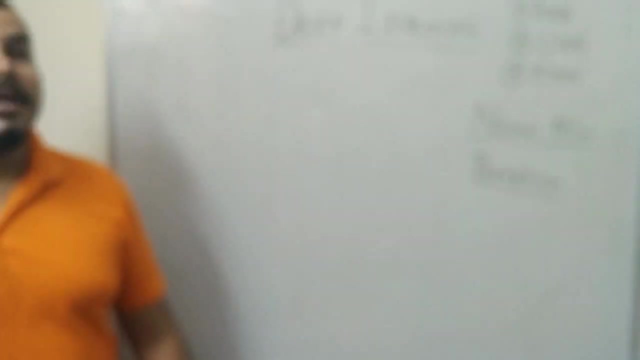 The first, simplest type of Neural Network was something called as Perceptron Perceptron. But there were some problems in the Perceptron because the Perceptron or the Neural Network were not able to learn very properly, you know, because of the concepts that were applied. 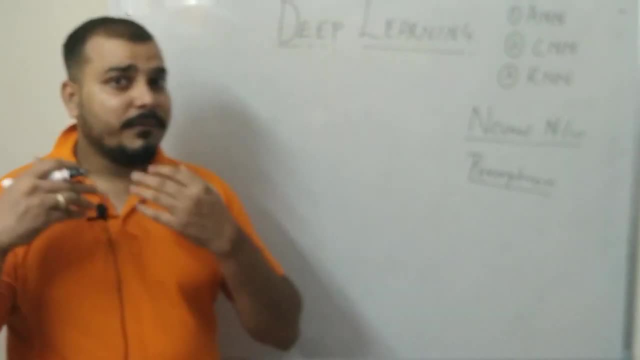 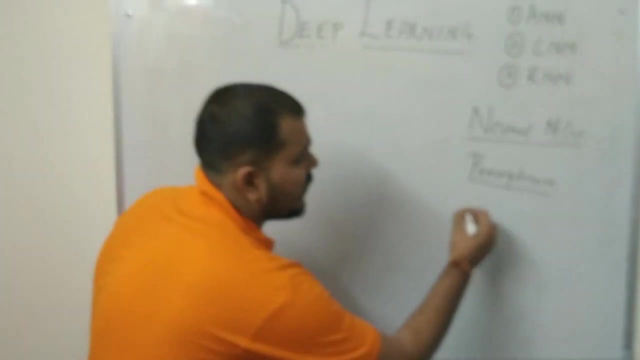 But later on, in 1980s, a researcher or a scientist or a teacher, you know, came up with a concept called Perceptron, But later on in 1980s, a researcher or a scientist or a teacher- he is basically my teacher also, because I have learnt lot of things from him- who is basically called as Geoffrey Hinton. 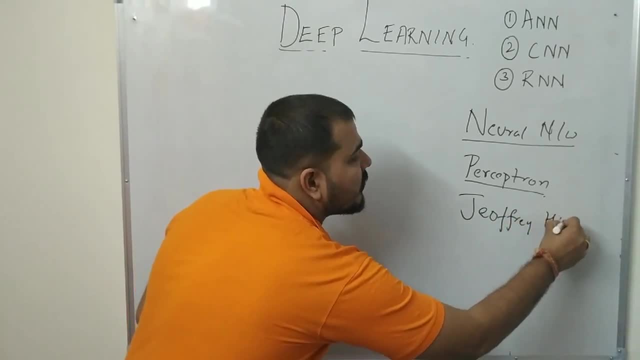 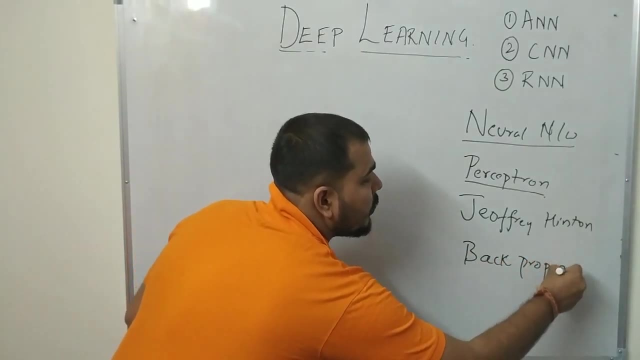 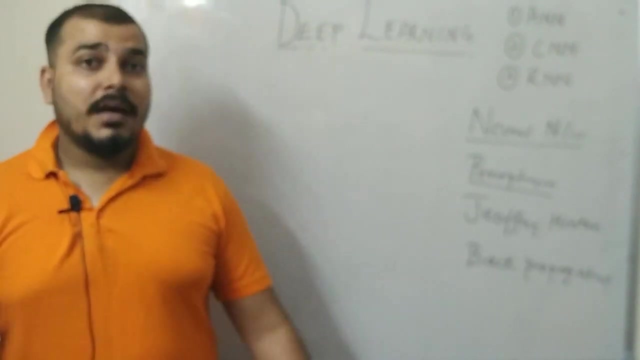 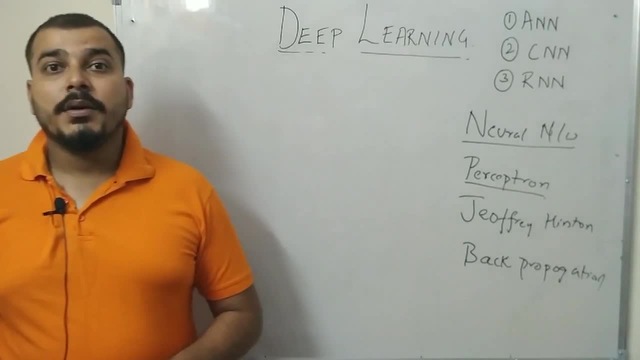 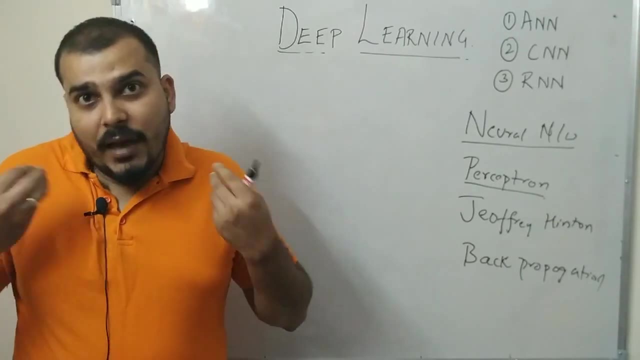 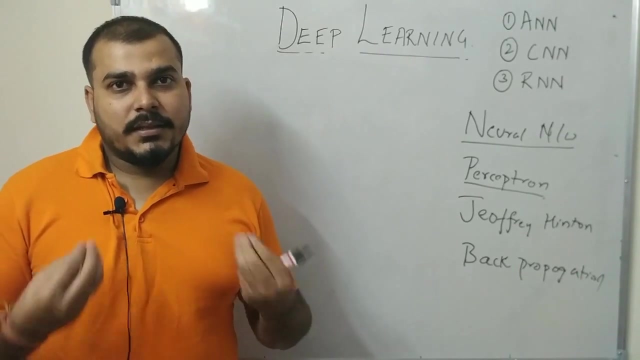 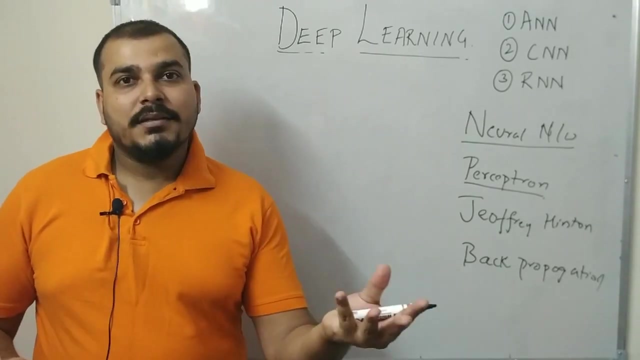 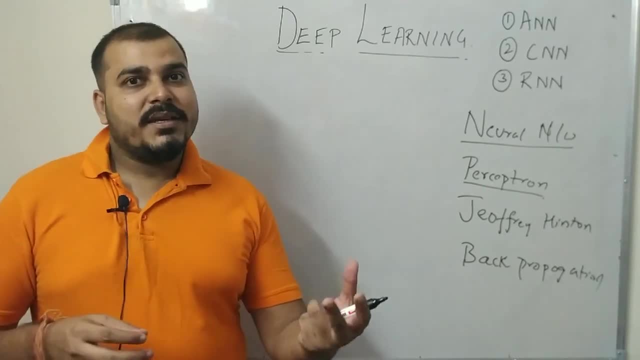 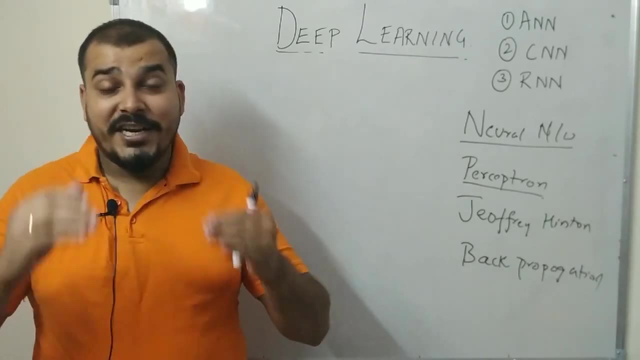 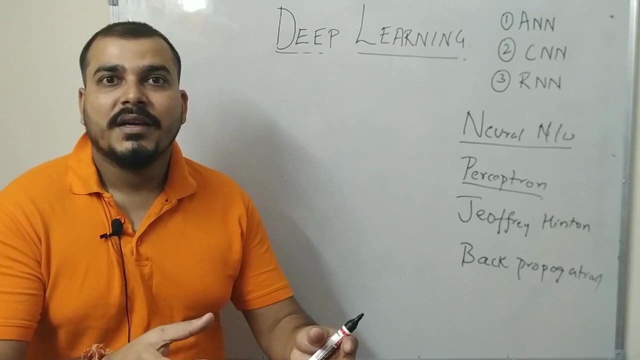 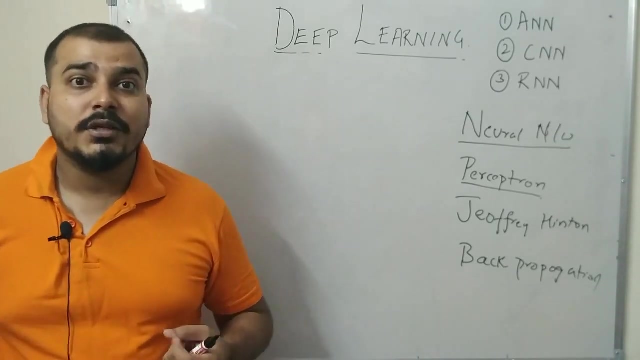 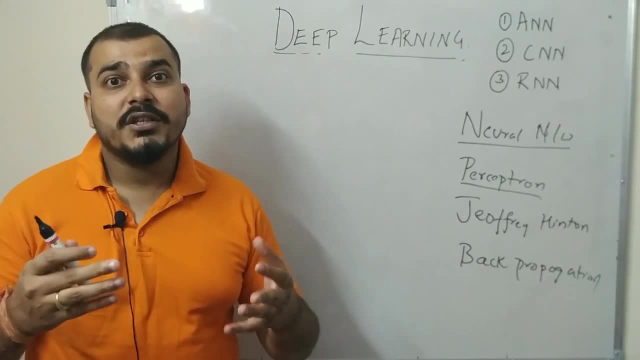 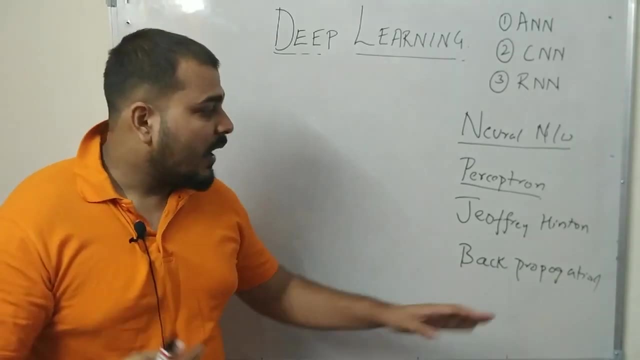 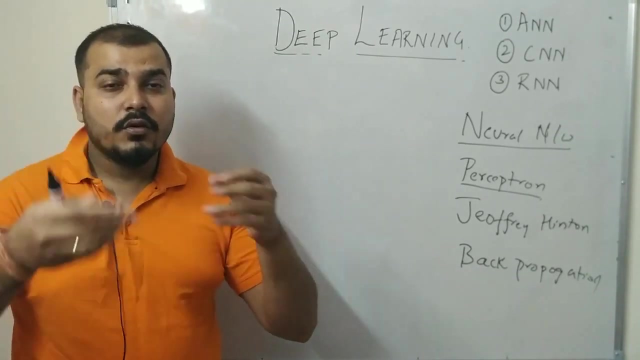 you know, by providing those features, ingesting those features, and each and every neuron present in that neuron network will learn those information and actually give you the output and with the help of back propagation also, it can train itself to learn new things. So to begin with, see, as I am ingesting the features through my sensory organs currently, 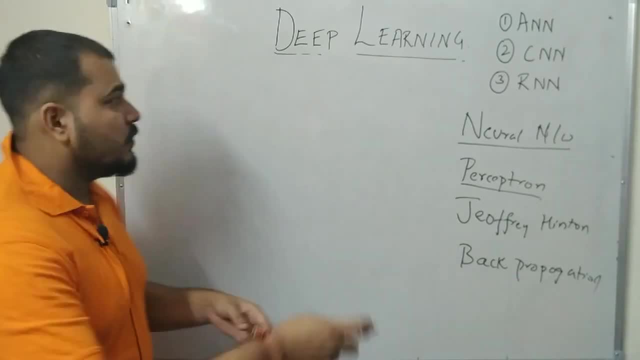 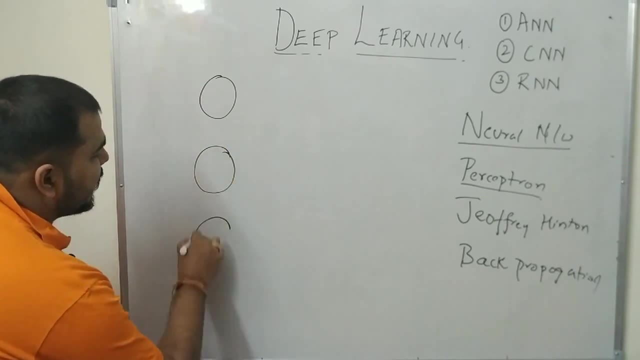 it is my eyes. so that layer is basically my input layer. So here the first layer of the neural network is basically the input layer. Now, input layer will have this kind of nodes which indicates that if there are features present in this. So these are my feature 1, this will be my feature 2 and this will be my feature 3.. 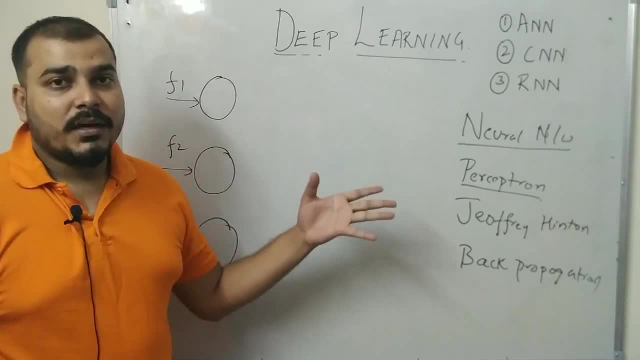 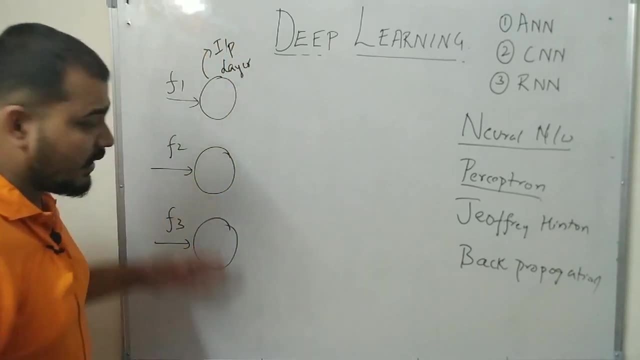 Suppose 3 features. I am trying to provide this to my neural network architecture, so this becomes my input layer. Now over here, in this particular example, I am actually providing 3 features and it can have any number of features over here. Then my second layer, after that particular information is passed through my eyes, right. 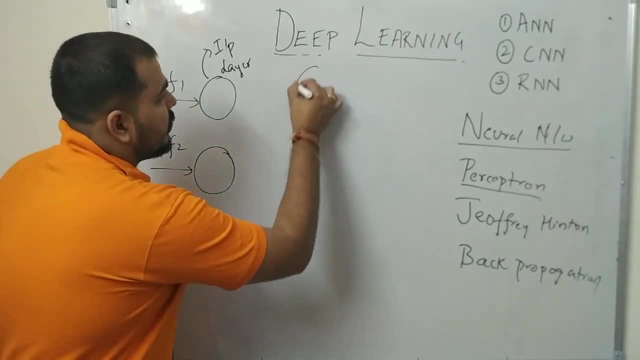 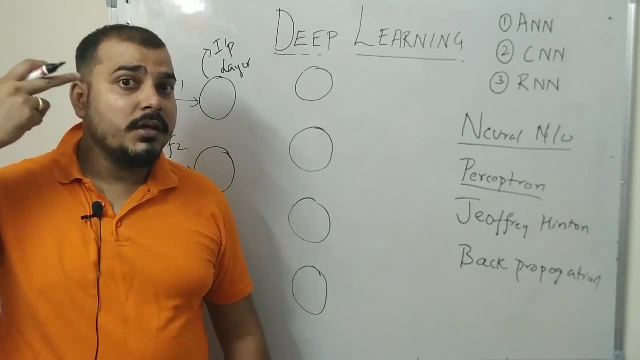 it reaches the hidden layer. So this is my input layer. Now hidden layer can have any number of neurons because- see now hidden layer, all this information from my eyes is getting passed through all the neurons. there is some pre-crossing happening in the neurons, but it passes through layers and each layer it can have any number of layers. 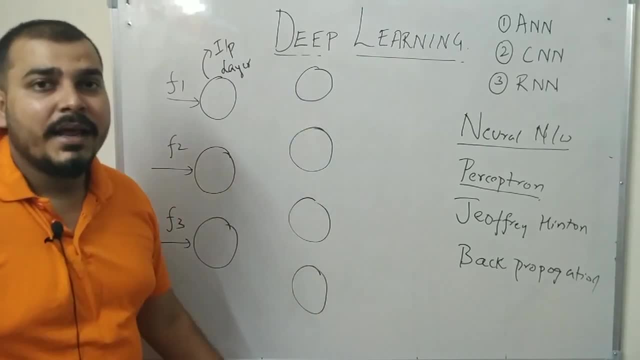 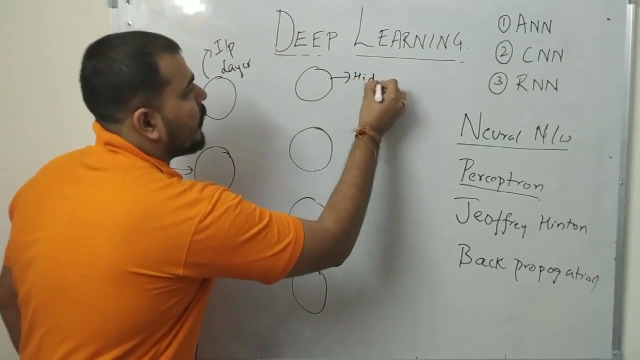 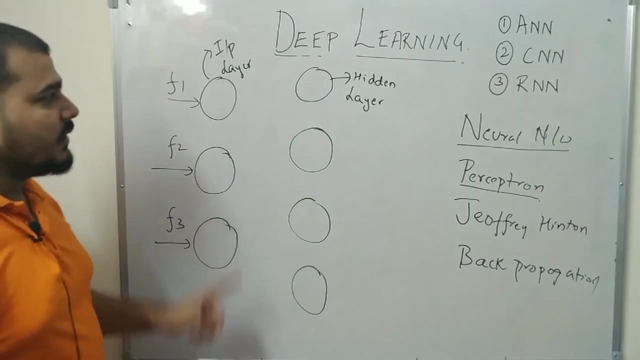 here for just simplicity and, for example, I am just drawing one hidden layer with 4 to 5 neurons, but it can have any number of neurons also. So this layer is basically my hidden layer. So this will be my hidden layer, and these all are neurons. 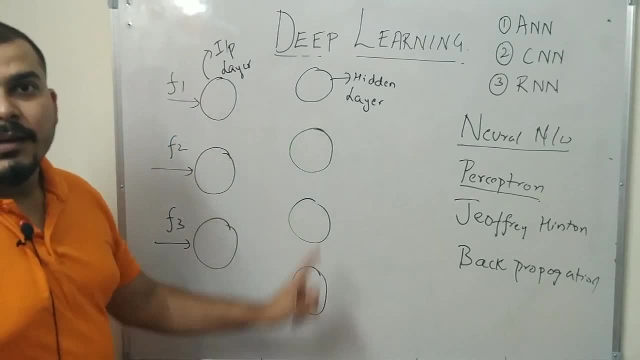 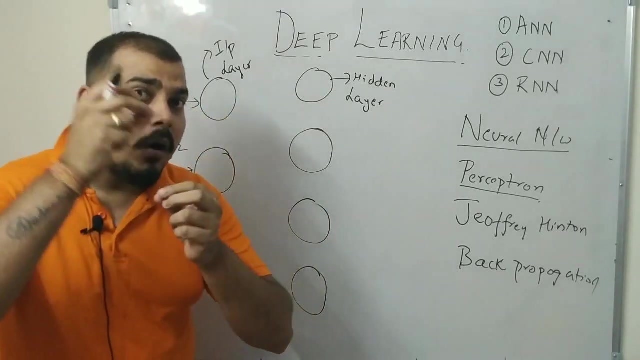 This, I will say it as nodes, this, I will say it as neurons, because these neurons are very important, because there is a lot of processing that is happening in these neurons which I will explain you in the next video of this particular playlist. on it, Then, remember, as the information, as the feature passes through my eyes, it goes through all. 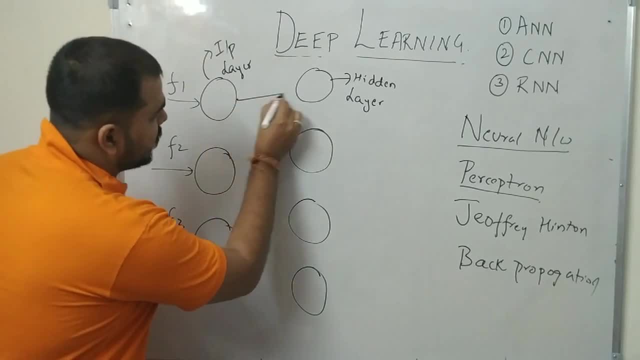 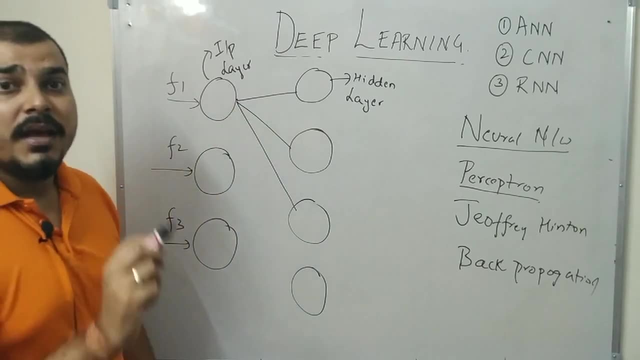 the neurons, right, get passed through all the neurons. So these features will get passed through all the neurons, and this particular line is very important, guys. So, because I will explain you what this is, This is what this line actually specifies. everything will be explained as we go ahead. 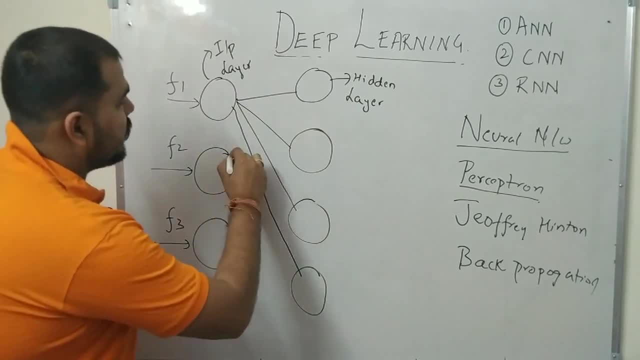 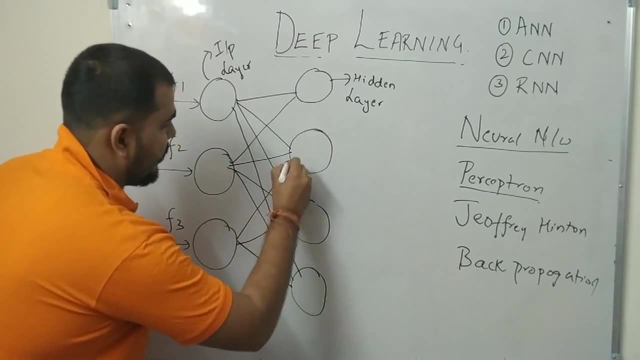 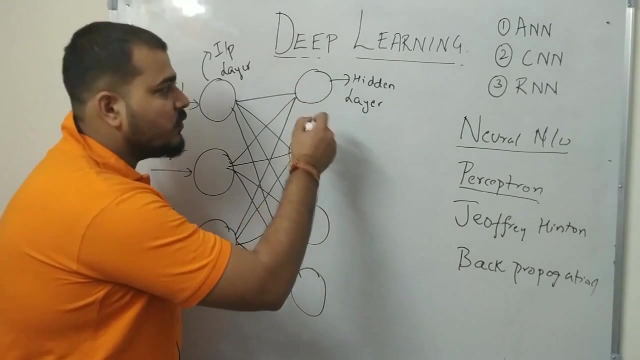 with this particular playlist. So this particular information passes through all the neurons- simple, all the neurons, right? So this all information is getting passed through all the neurons in the hidden layer, and then some kind of pre-crossing happens over here and then finally we get the output. 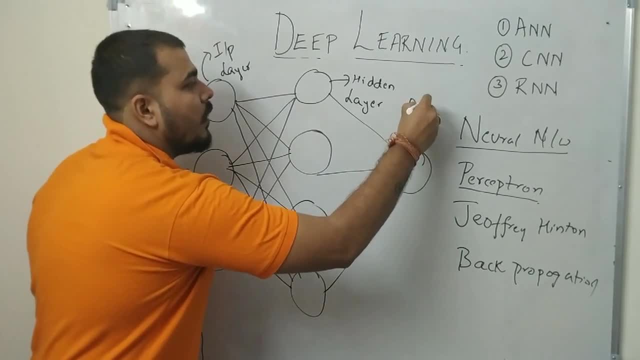 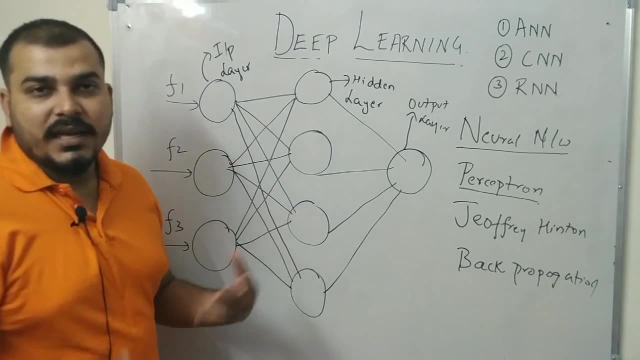 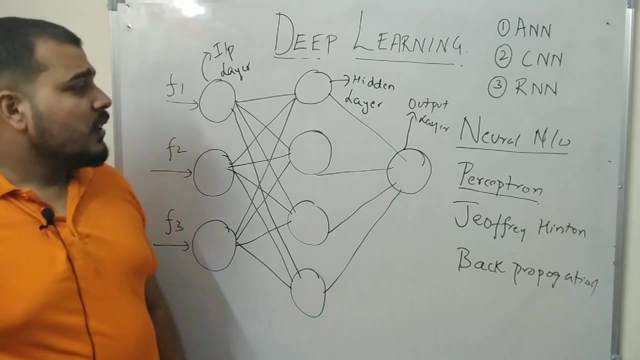 And this is basically my output layer. It can be any number of outputs. also I can draw multiple. suppose it is a multi classification, that many nodes I can create. if it is a binary classification, then I need to just specify one node over here which, basically based on probabilities, you will be basically getting. 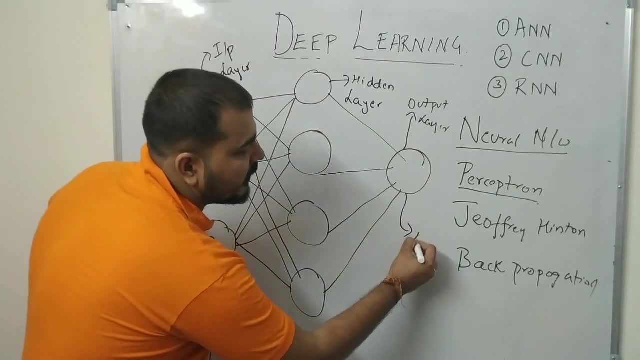 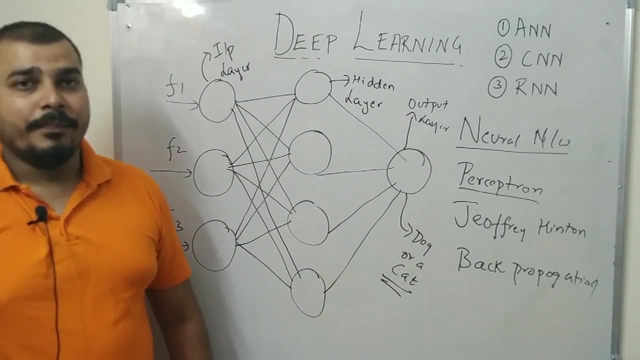 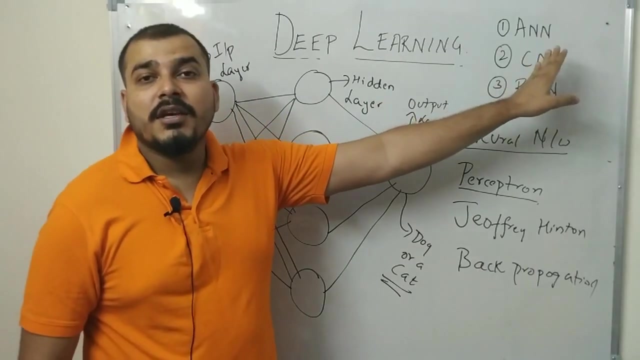 what is the output? and this particular output will specify whether that object is a dog or a cat. right, and this is basically called as your output layer. So this is the simple neural network architecture, and when I say neural network architecture, this actually resembles something called as artificial neural network, combination, neural 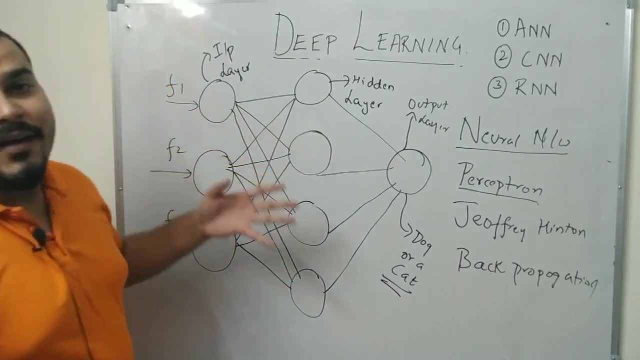 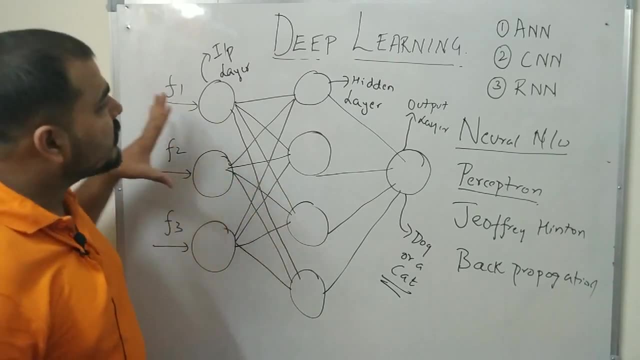 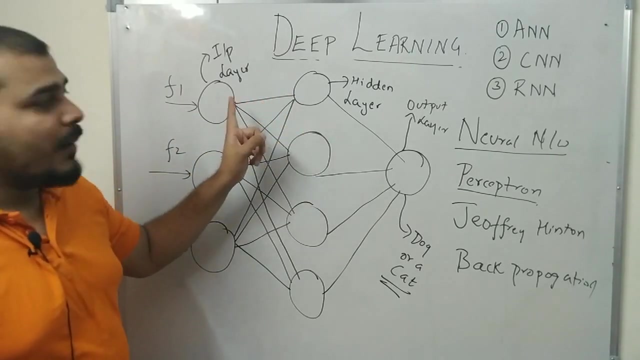 network has a different theoretical concept. it will also be having this kind of neural network, but you will be having other layers also which I will be discussing in my future classes. but just understand, this is the basic neural network architecture of an ANM. Now in my next video we will try to understand these lines that are connected. what happens? 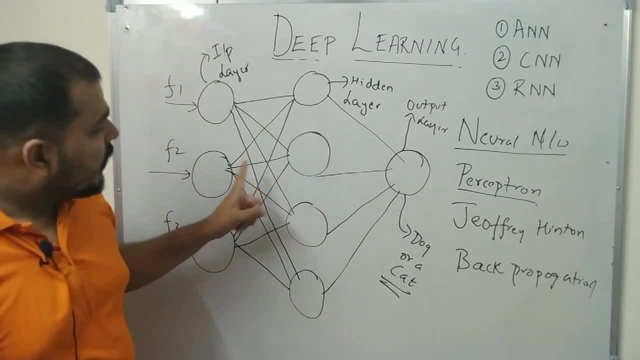 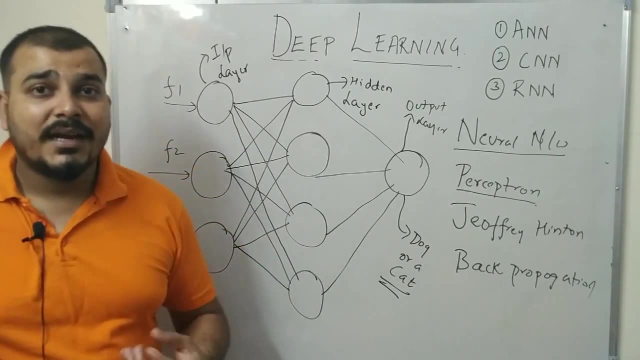 what type of pre-crossing happens in each and every neurons- okay, with respect to this, neurons that are present over there- and there is also concept called as activation functions. what is the use of that activation function? everything will be explained in the upcoming videos and we'll also discuss all the different kind of activation functions also.